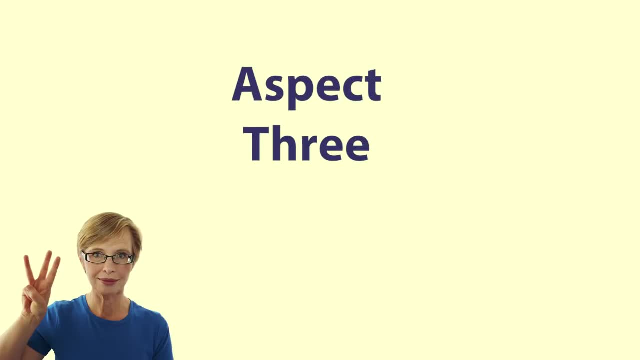 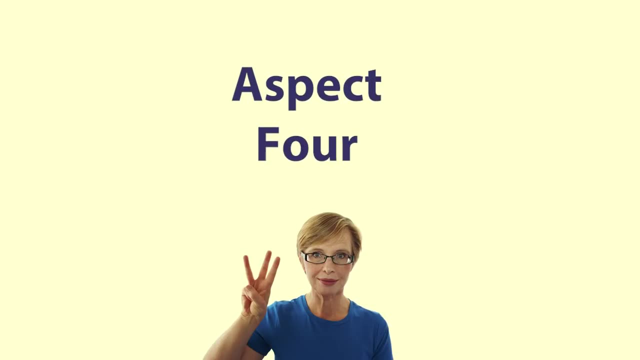 distribution. Aspect 3. The spread of the sampling distribution is related to the spread of the population values. Aspect 4. Bigger samples lead to a smaller spread in the sampling distribution. I will now illustrate these aspects with an example. We have a population of dragons. 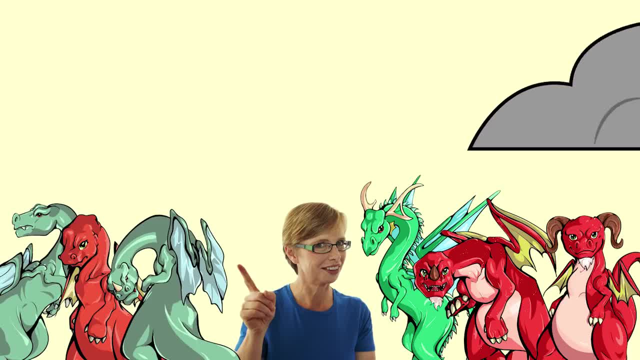 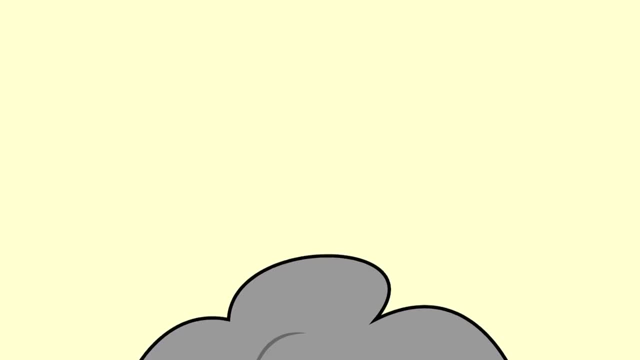 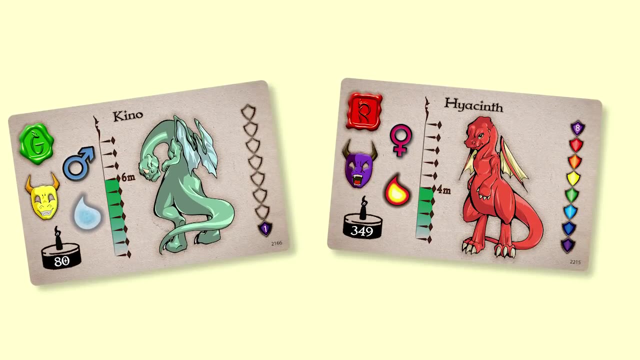 And we wish to know their mean strength in order to tell whether the change in climate is affecting them. We want to compare that with information from previous scientific studies of the dragons. Each dragon is represented by one of these data cards. From experience, we know that the range of dragon 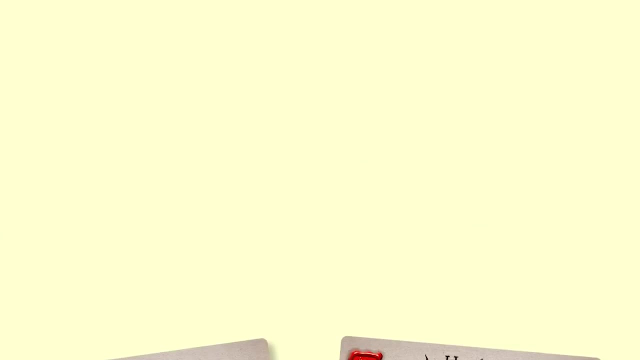 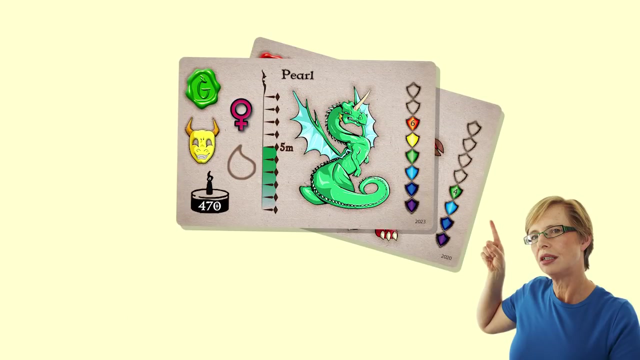 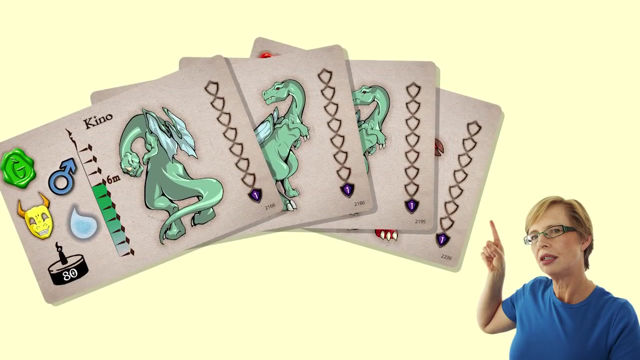 strengths goes from 1 to 8.. There are 720 dragons in the population and we're taking a sample of 4 dragons. These are very small samples but are useful for illustrative purposes. How likely is it that the average strength of the 4 dragons will be 1?? 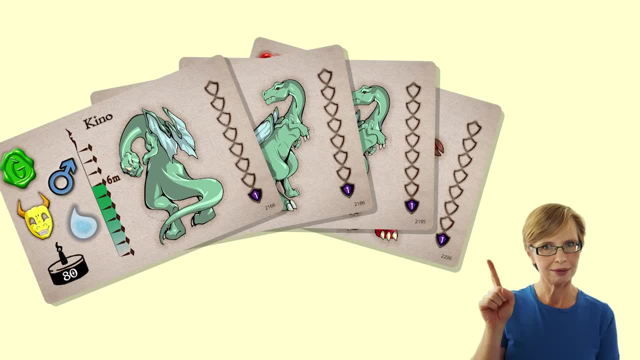 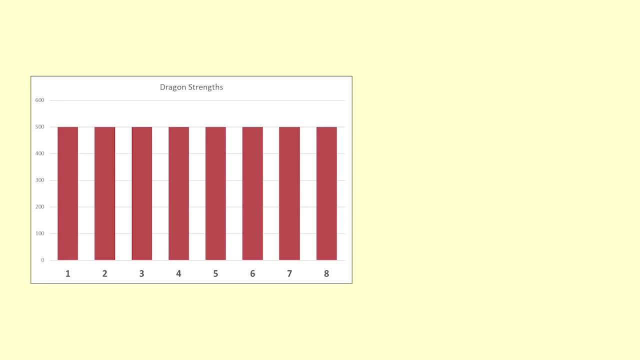 You are right. It is very unlikely. All 4 dragons would need to have a strength of 1 for the mean strength to be 1.. If there are equal numbers of dragons at each strength, then the probability of getting 4 dragons of strength 1 is 1 eighth to the power of 4, which equals 0.00024, or one chance in. 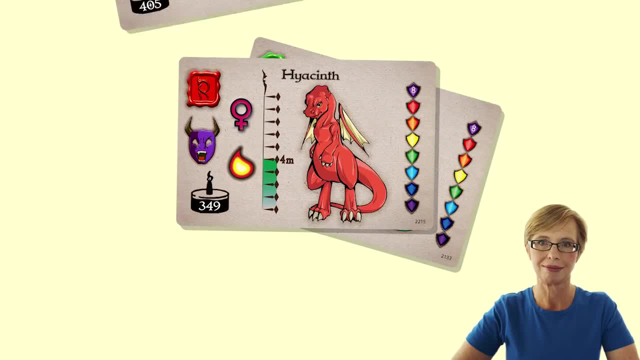 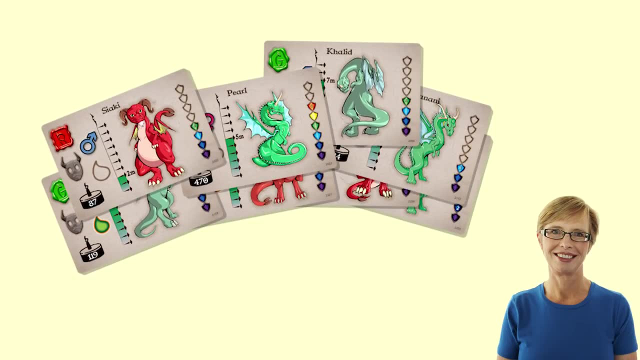 4096.. Similarly, it is very unlikely that the mean strength will be 8, as all 4 dragons would need to have a strength of 8.. Let us take some samples of our dragons and see what the mean strength is for each sample. 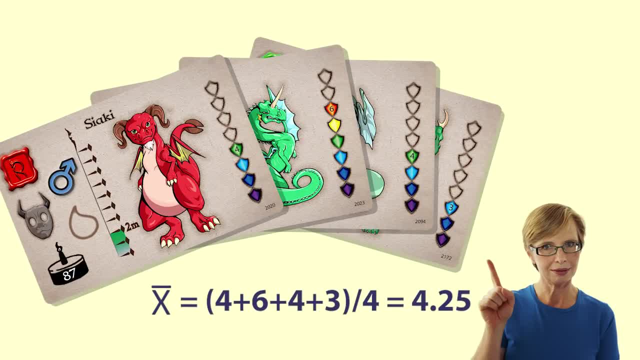 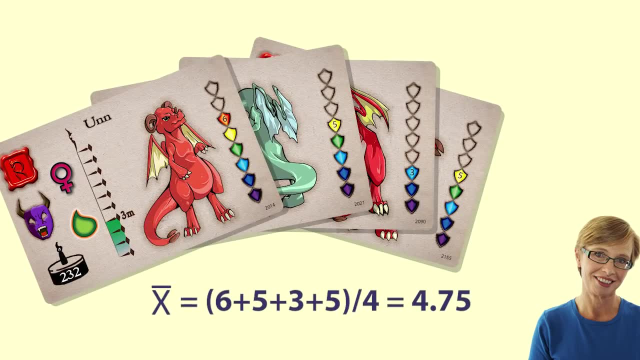 Here's our first sample. The mean is 4.25.. And here is another sample: The mean is 5.25.. And here's another sample: The mean is 4.75.. And here are a few more samples: The means are 6,, 5,, 3.35.. 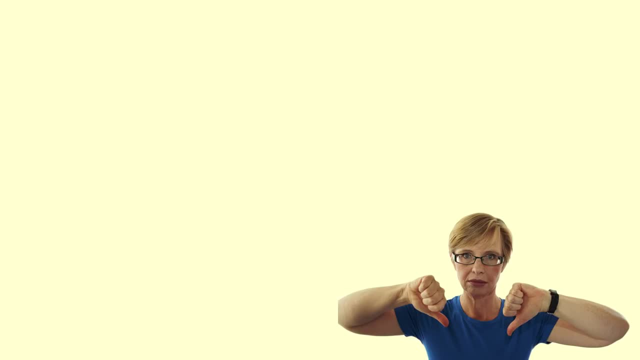 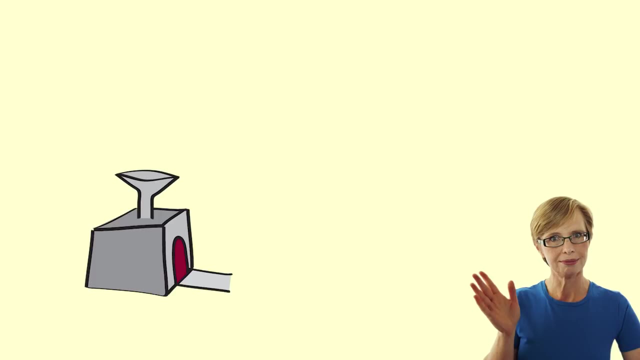 It could take a long time doing this by hand, so let's set up our computer to simulate taking 4000 samples of 4 dragons from our population. We can only do this because we happen to know all about the dragon's strengths, having. 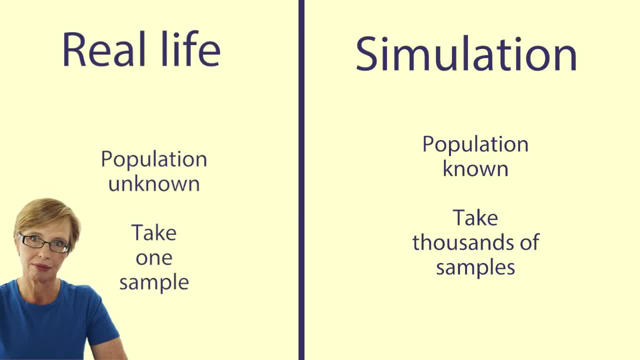 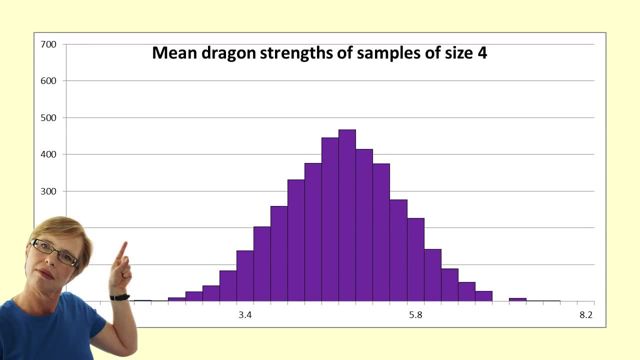 made them up in the first place. This is a simulation. we would never know this in a real life study. Here is a distribution of those 4000 means from samples of 4 dragons. Let's look at the 4 aspects mentioned before. 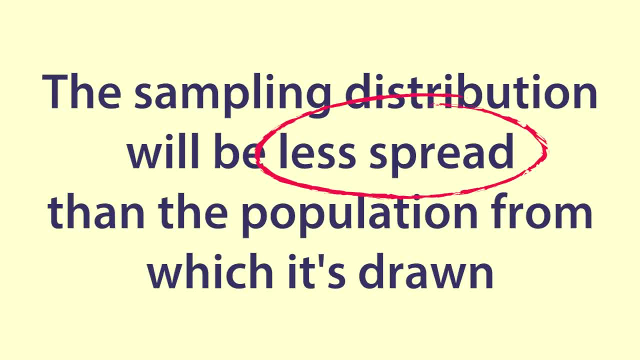 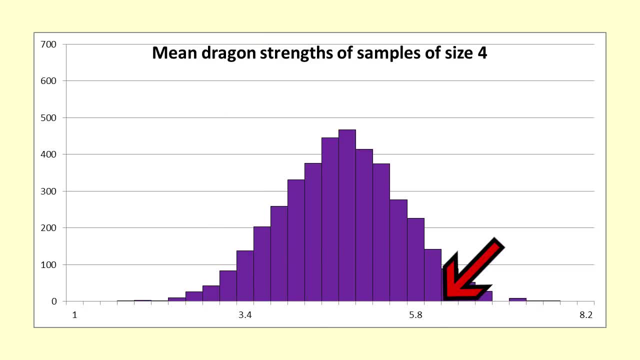 Aspect 1. The sampling distribution will be less spread than the population from which it is drawn. You can see that most of the sample means lie between 3 and 6, and all of them lie between 1.75 and 7.5.. 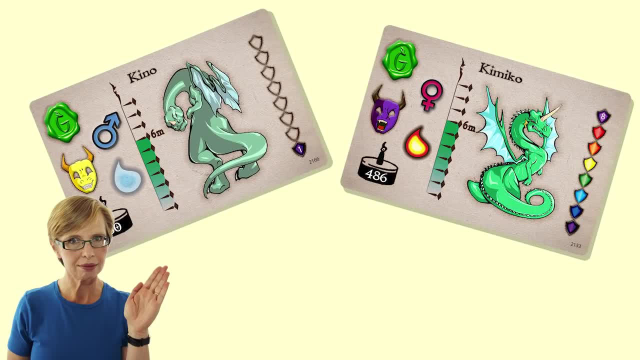 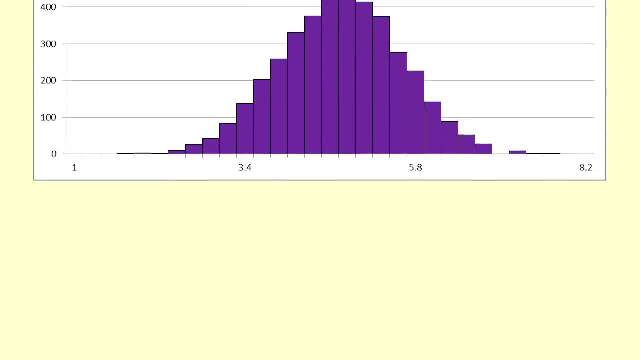 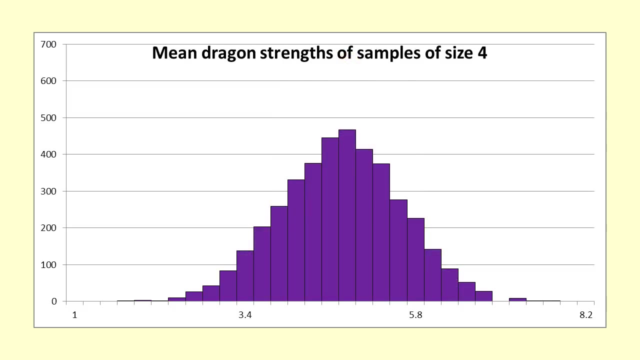 Remember the population values lie between 1 and 8.. Aspect 2. The sampling distribution will be well modelled by a normal distribution. You can see that even with samples of size 4 that the distribution resembles a normal distribution with a bell shape. 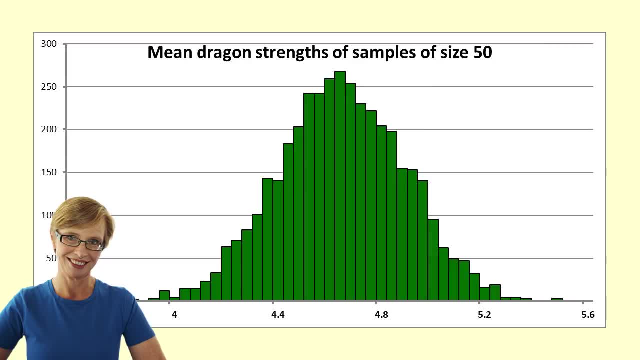 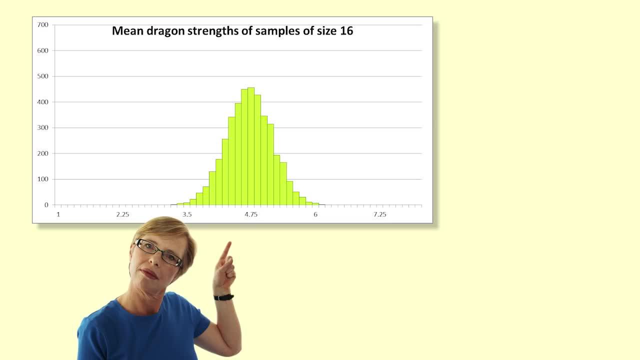 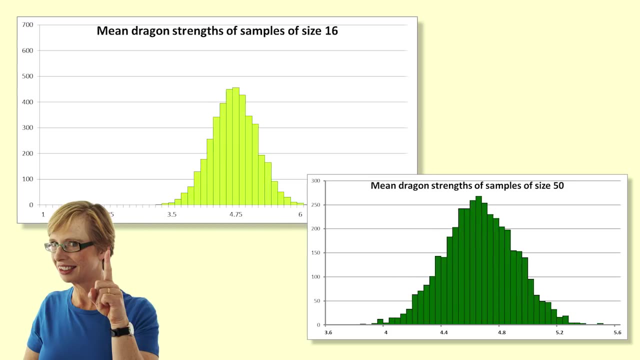 If we take larger samples, the distribution gets closer in shape to a normal distribution. Here are graphs showing the spread of sample means of dragons from samples of size 16 and 50. You can see that the shape is getting more like the normal distribution. 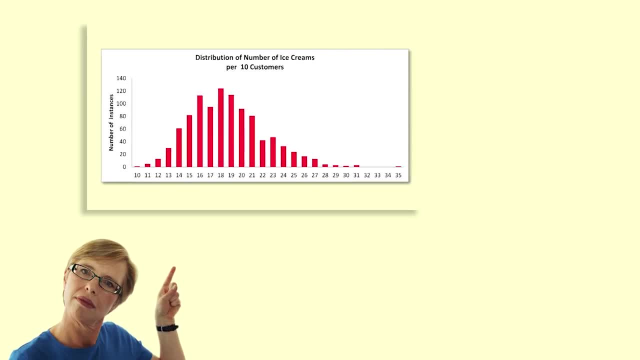 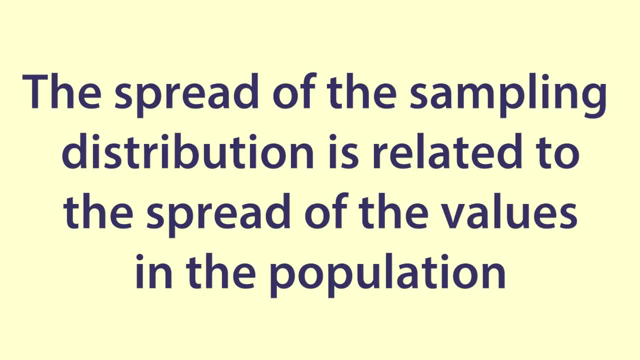 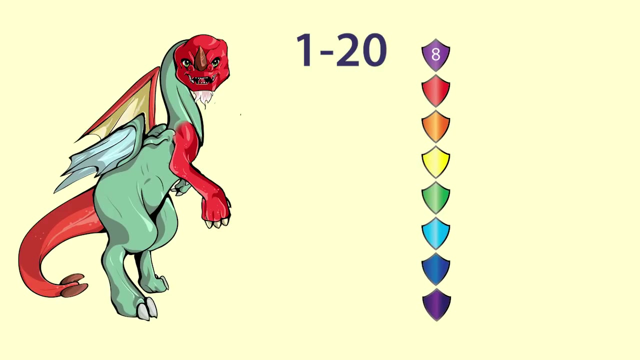 This is also shown in our video about the normal distribution, Aspect 3.. The spread of the sampling distribution is related to the spread of the values in the population. Say, a different dragon population had a spread of strengths of 1 to 20 instead of 1 to 8.. 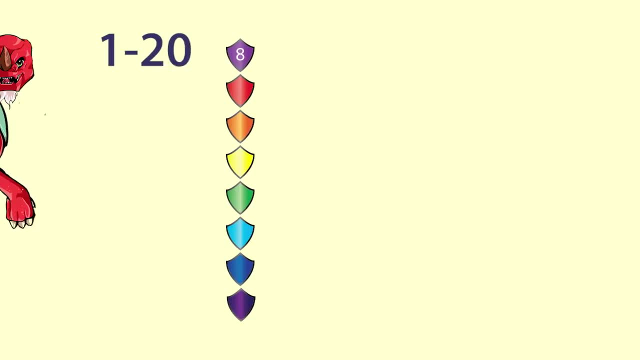 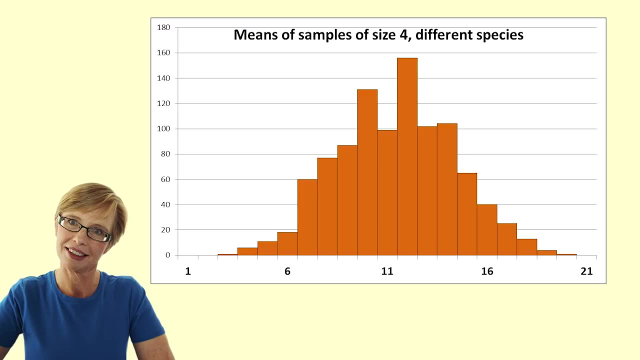 You would expect the spread of the sample means to be greater. Here is a graph showing the spread of sample means from samples of size 4 from a different population of dragons. These dragons have strengths evenly spread between 1 and 20.. Aspect 5.. 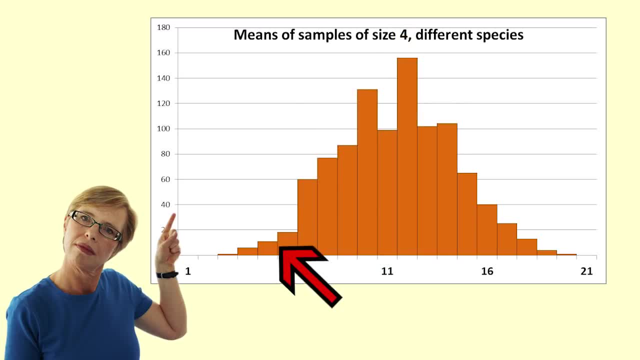 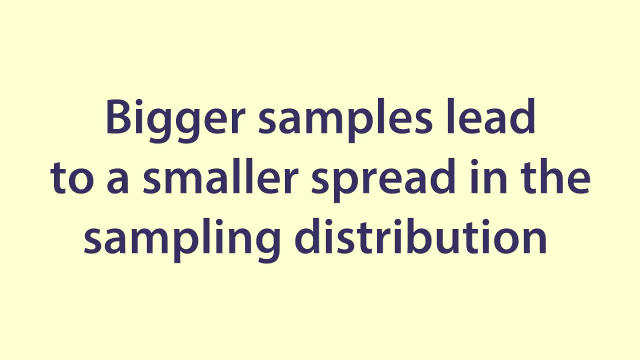 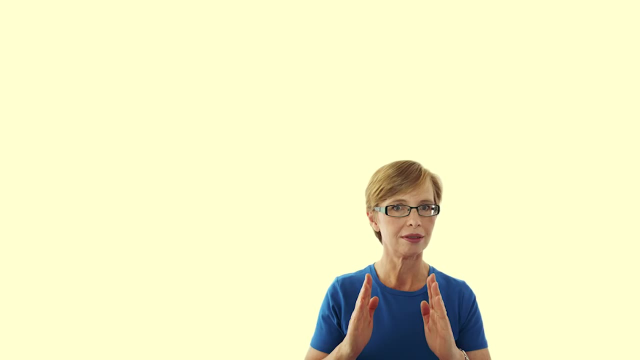 You can see that there is still the bell shape. Aspect 6. For these dragons, most of the sample means lie between 6 and 16.. Aspect 4. Bigger samples lead to a smaller spread in the sampling distribution. The bigger the sample, the less likely it is that all of the values will be small or 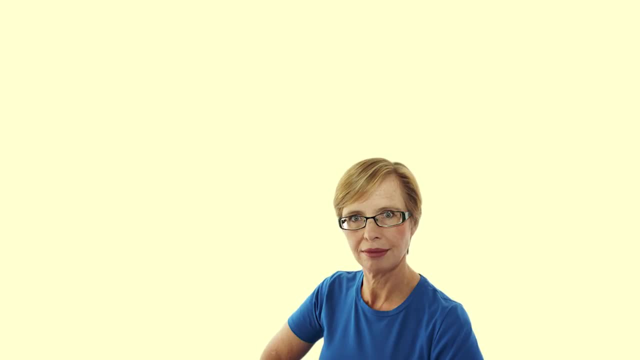 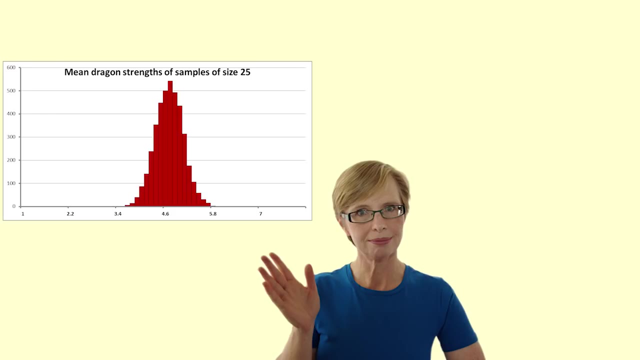 that all of the values will be large, so that the chance of extreme values is reduced. Here is a graph showing the spread of sample means of strengths of dragons from samples of size 25.. And here is a graph showing the spread of sample means from samples of size 25 to 1..